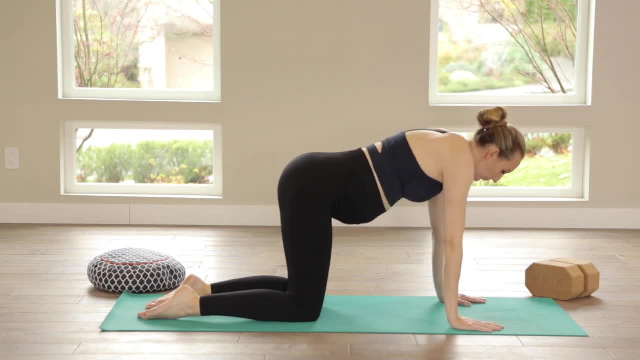 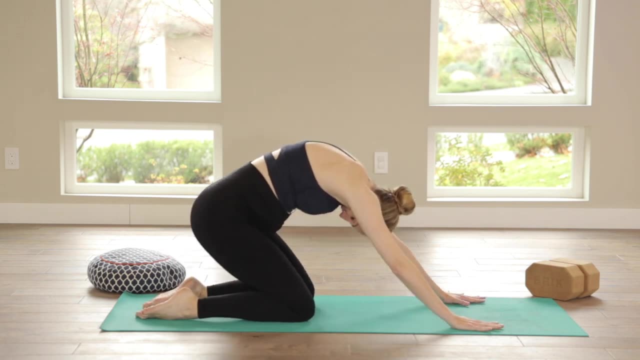 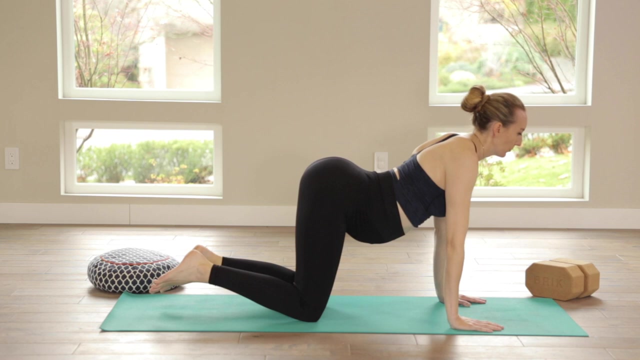 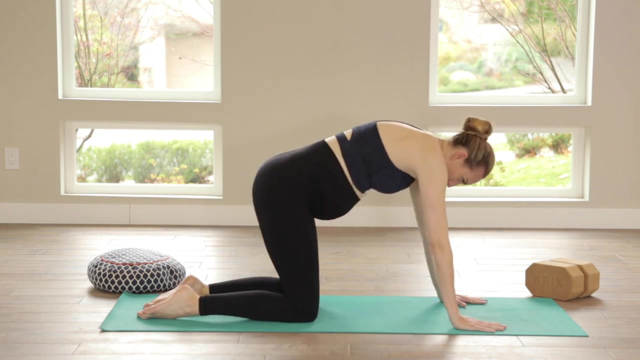 Moving deep within the womb, slowing down your breathing- Really nice- And then coming back up into a table pose. A lot of times the reason our low back hurts during pregnancy is because it's not carry all the weight we have in the front of the body. 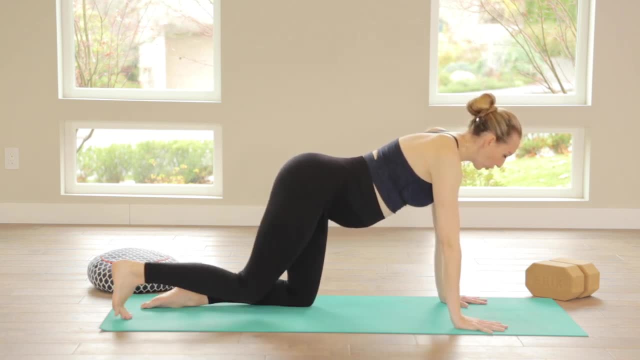 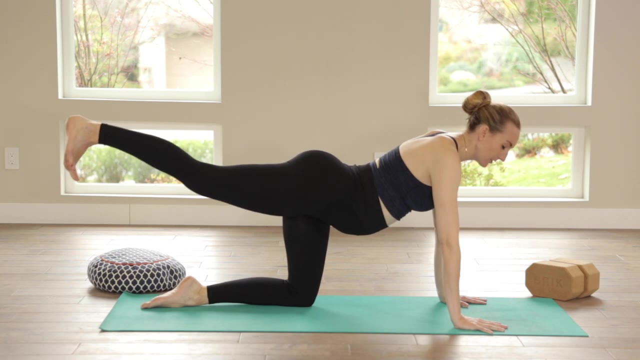 So spread the fingers wide, curl your right toes underneath you, so your right leg's gonna come straight. and then I want you to lift your right leg up off your sticky mat. As you do that, hug baby in, So right away you'll feel your low back muscles. 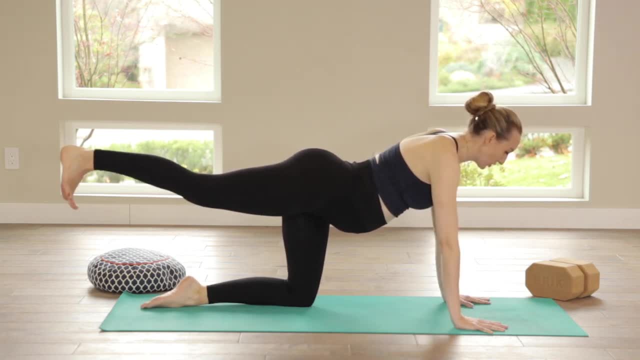 a little bit start to turn on. So what we were just doing was stretching. now we're gonna do a little bit of strengthening. So option one: just hold here. Think of your right inner thigh moving towards the ceiling and your pinky toe moving down on the right leg. 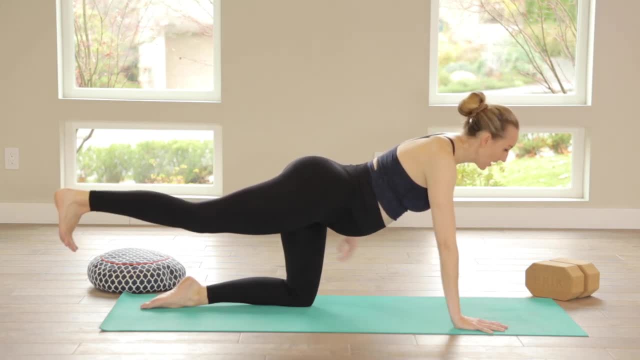 So it almost feels like your right leg's kind of quirk screwing into the body And then maybe you feel that low back, turning on And deepen the breath And then option to just hold here or reach the left arm out. So these aren't our favorite exercises. 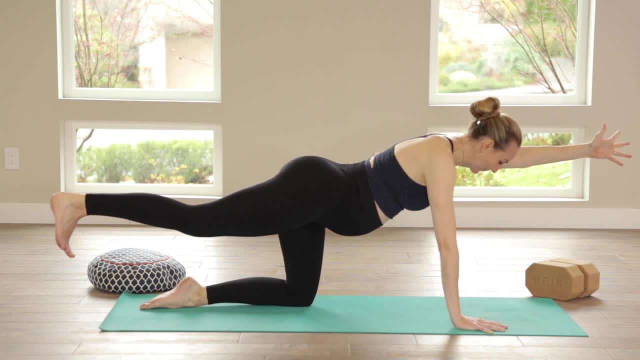 but they're so good for us. Keep hugging baby in So you don't need to lift the left leg off the ground. just holding this right leg up behind you, especially in third trimester, is plenty, Those of you who've been doing this routine for a while. 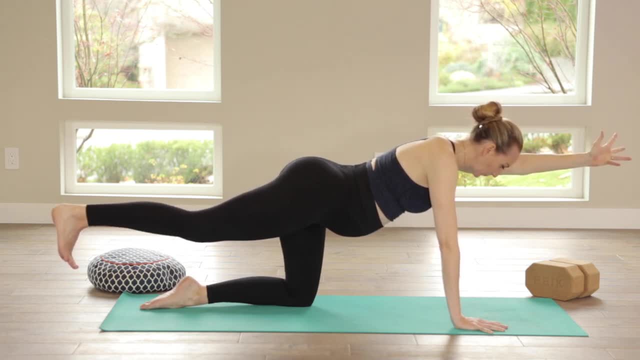 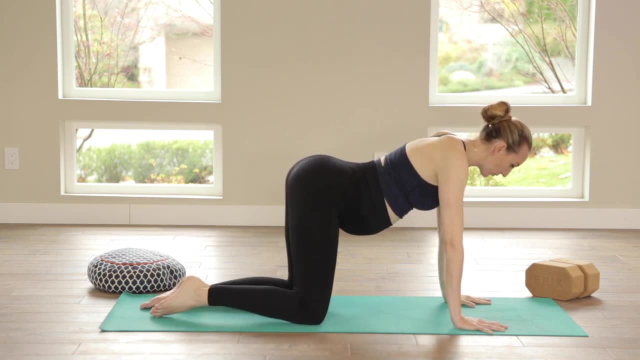 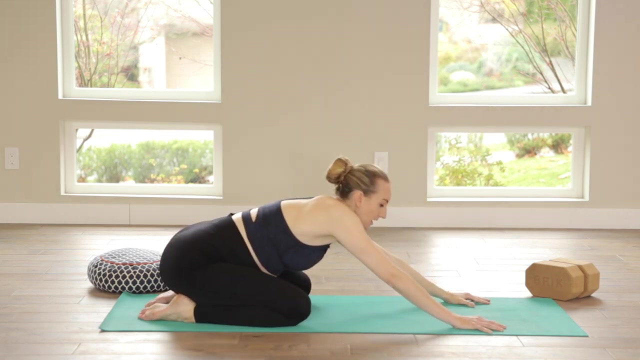 and are building up that strength. reach the left arm forward, Keep deepening the breath, Good- And then set that right knee down. Let's do some juicy hip circles. So take the knees a little bit wider apart, shift the hips all the way over to the left. 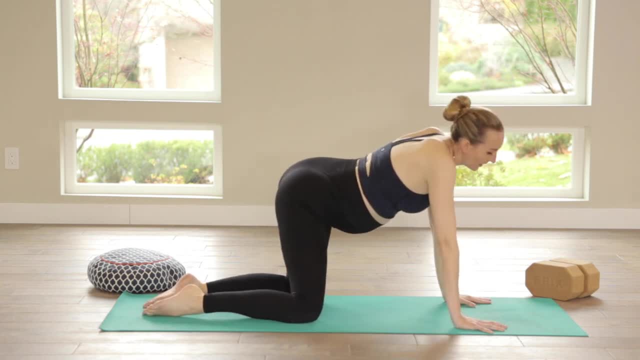 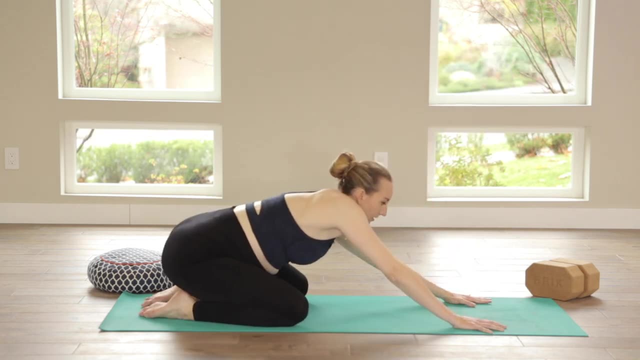 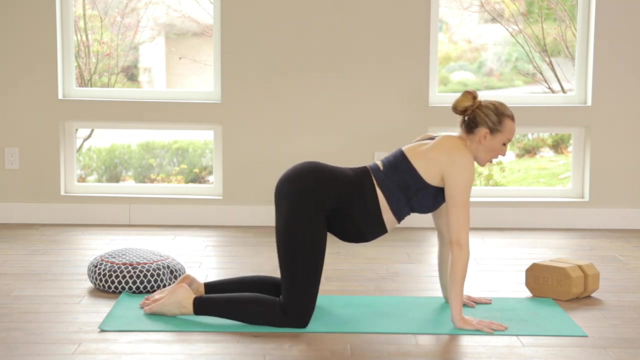 feet to heels, hips to the right And just add some lubrication to this area of the hips and the low back. Okay, So we'll do that little low back strengthening exercise on the left And then we'll come into some more juicy stretches. 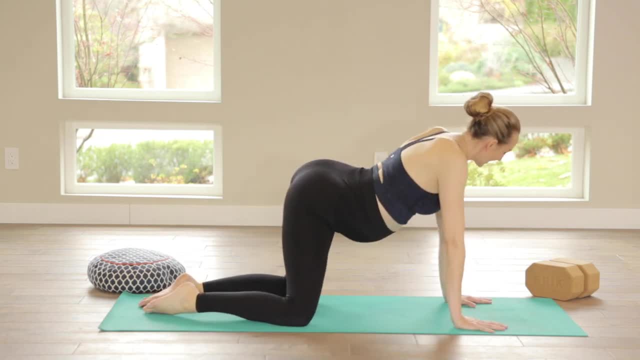 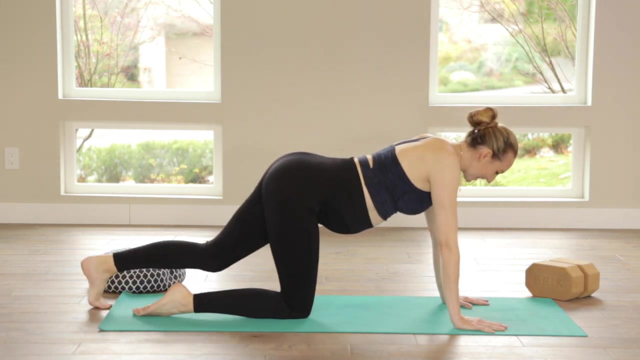 What I've found over two pregnancies is that we need to strengthen. Stretching's important, but we need to strengthen too to support all this extra weight of baby. Come back to the hips: directly under the knees, Knees directly under the hips. extend the left leg back. 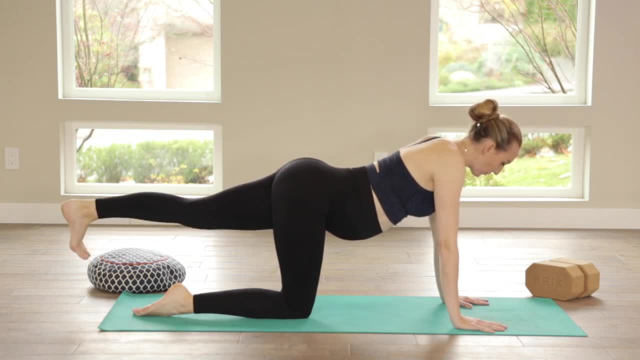 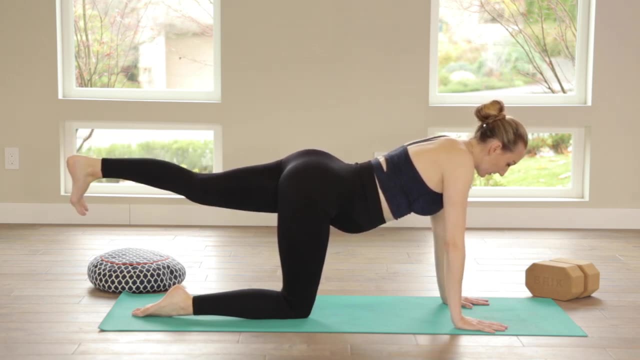 And from the inner thigh. so think of moving from the inner thigh and your pinky toe moving towards your sticky mat. lift the left leg, Hug baby in, so draw navel to ceiling so you're really snuggling baby up into you and 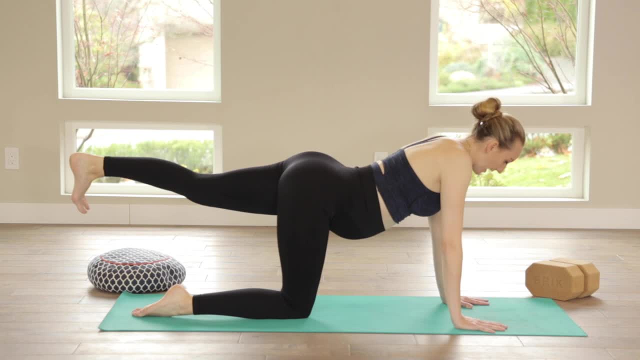 hold here. It's subtle, but you should feel the left side of your low back activate those muscles. turn on, You choose the intensity level so you can stay right here or you can lift the right arm if you want a little bit of that extra challenge. 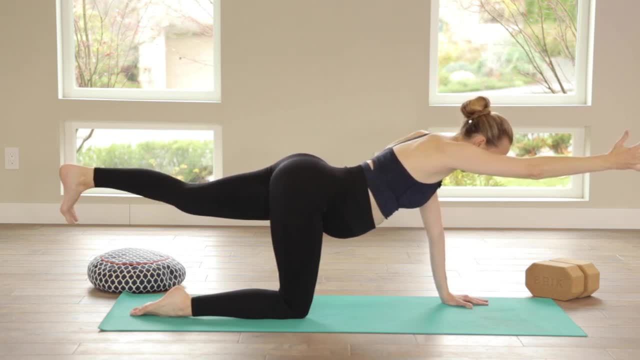 Deep in the breath- which is great practice for labor as well- where we're going to be dealing with maybe some discomfort or sensation- I like to just choose to call it sensation- but we can use our breath to ride, navigate, surf the wave of that sensation without getting 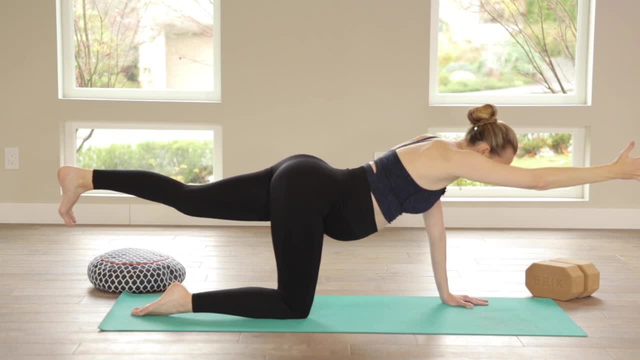 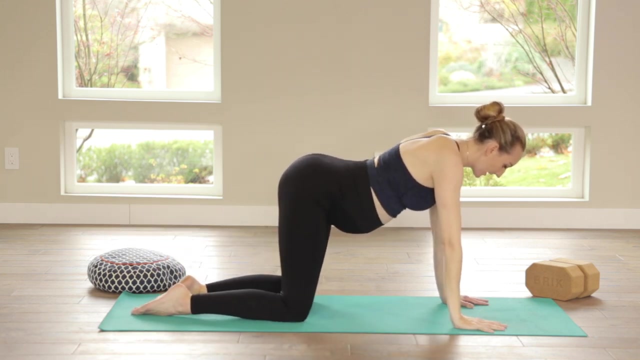 flustered, Hug baby up. and in Last three, two: keep that back left foot super flexed. last one: good, Take the hand and knee down, widen the hips a little bit or widen the knees a little. 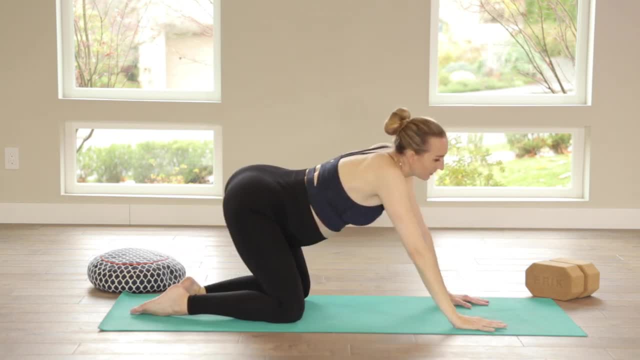 bit and we'll do those big hip circles again. So I really want you to think of your hips moving almost off to the side like so much, because that's going to give you a little bit more flexibility. So we're going to do a little stretch here in the outer hip- beautiful. 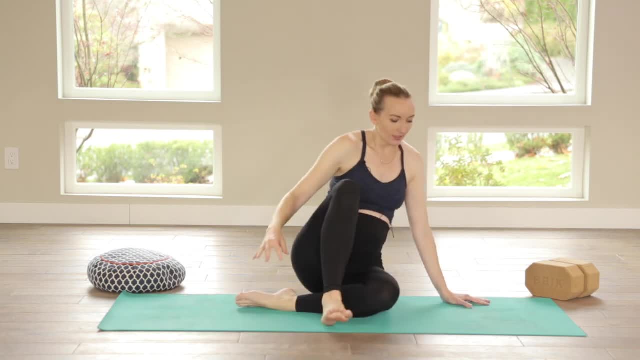 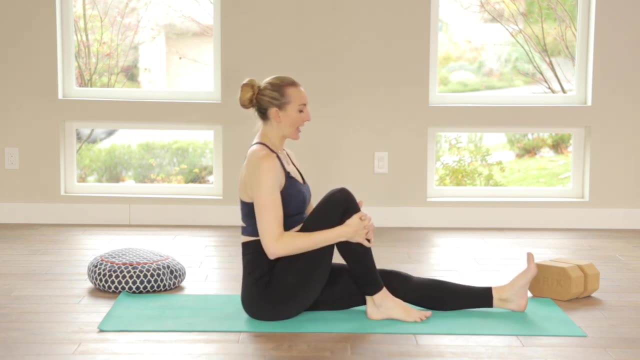 All right, let's come to sit. Take your legs out in front of you. We're going to come into a half butterfly stretch, So pull your right knee up into the chest. The left leg is long, with the foot flexed and active. 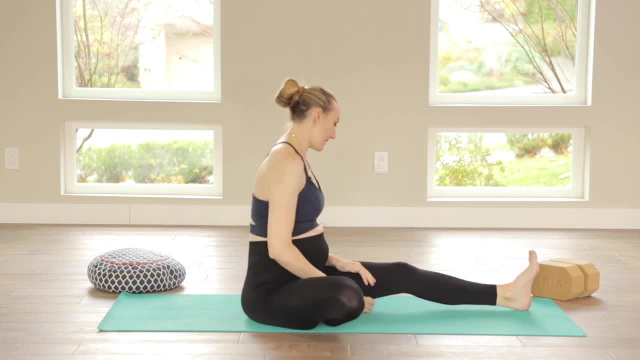 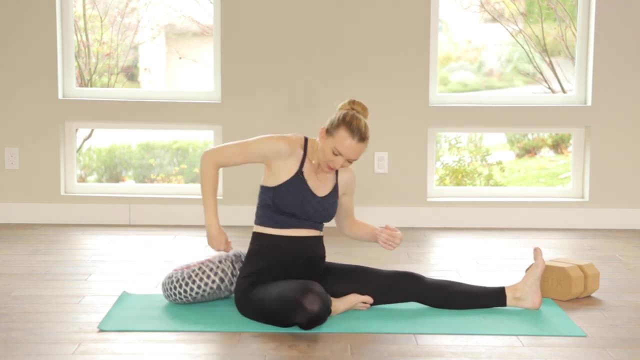 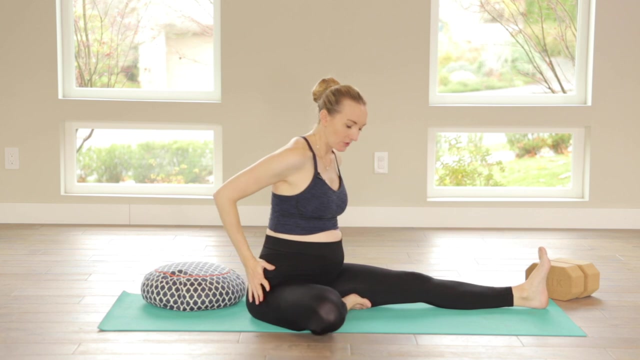 Open up the right knee. Take the sole of the right foot into the inner right thigh. Now, if you need to sit on some blankets or even a cushion in this position right to get comfy, it's all good. So, couch, cushions, pillows, all work. 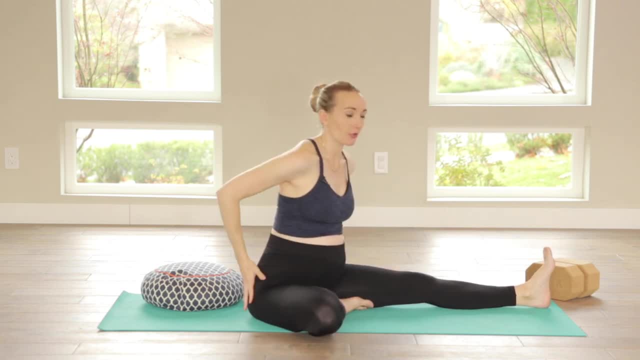 This is a great position for third trimester pregnancy. This is called Janu Sirsasana. Inhale, reach the arms up and then exhale. just fold over your leg, resist the urge to grab the foot. So I'm actually going to have my palms facing down on the mat, as you can see, and then I'm. 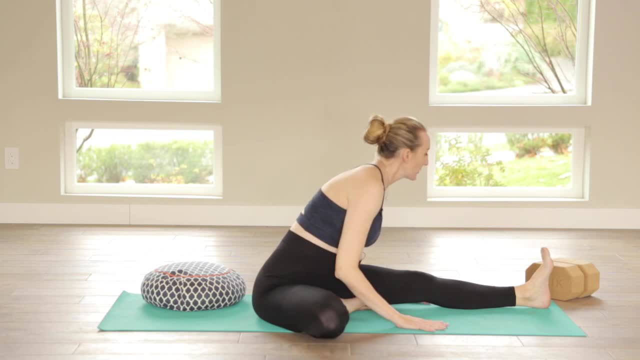 going to slide my shoulder blades down my back. We don't need to focus on flexibility right now, because relaxin, this hormone developing in our body to prepare us for labor, is already making us more flexible than we need to be. So instead, here it's less about holding the foot. instead, I'm drawing the shoulder. 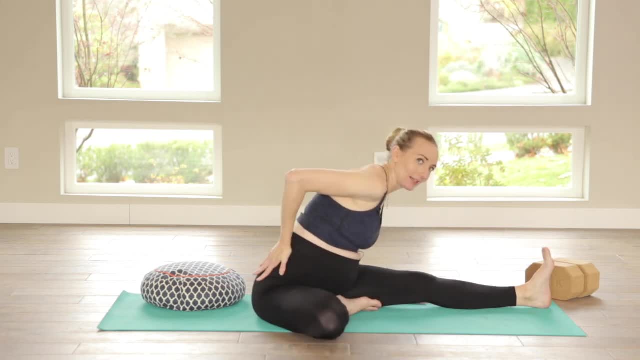 blades down and I'm more interested in what I'm feeling in my low back. all right, So two breaths here and I'm going to show you a couple variations. So nice to have a little stretch on the back of the left leg, but again I'm not reaching. 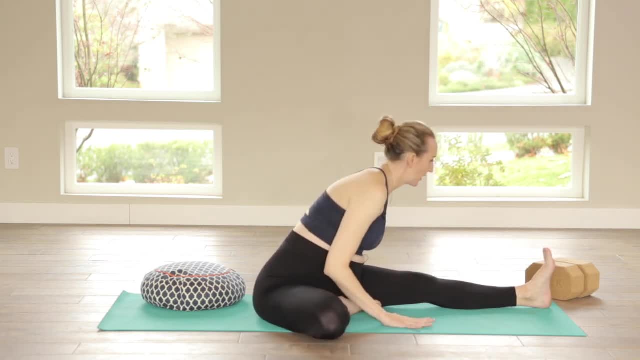 or pulling or, you know, rounding forward to try to get the foot. I'm really focused on sending my breath into the sacrum, low back area. beautiful, Slowly, press yourself up. good, and now we're going to adjust this. take your hands behind. 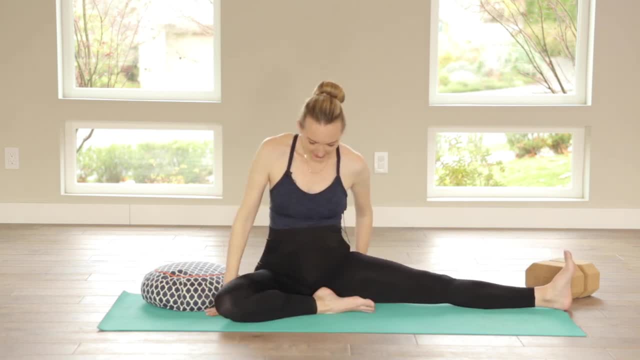 you. So you're going to press this. you're just going to come into a little bit of a more open hip position So your heel might move a little bit closer towards your groin, or not. Keep the left hand on the left thigh so you'll be doing the reverse of me if you're watching. 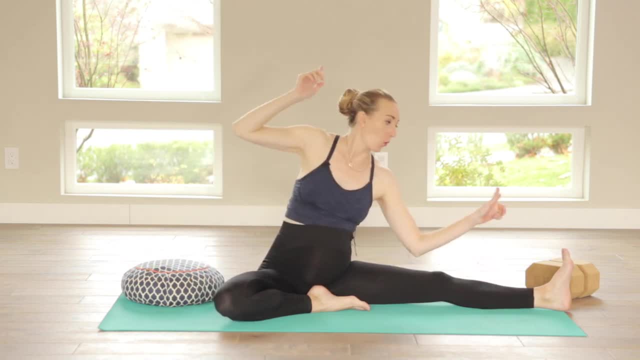 the video. Take the right arm up and you're just leaning towards that leg, okay, And then what I like to do here is actually take this top hand and cup it underneath my face, So I'm kind of holding my ear. I feel like an ear muff. 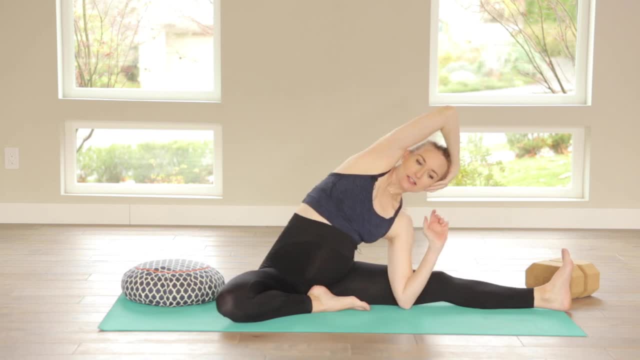 And then sending my elbow up and back And then this on the bottom hand elbow can rest either on my thigh or on the floor. Sometimes I like to hold my ankle and then I think of my heart spiraling towards the ceiling. 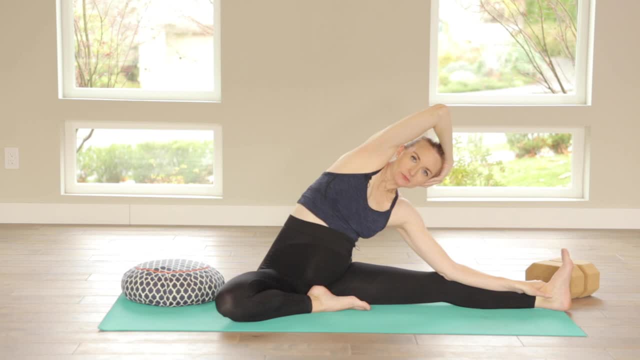 Three deep breaths here. Let the hips be really heavy. Good, Good, Two more Good. So the next thing we're going to do is kind of get our hands together and then we're going to be doing some plank. 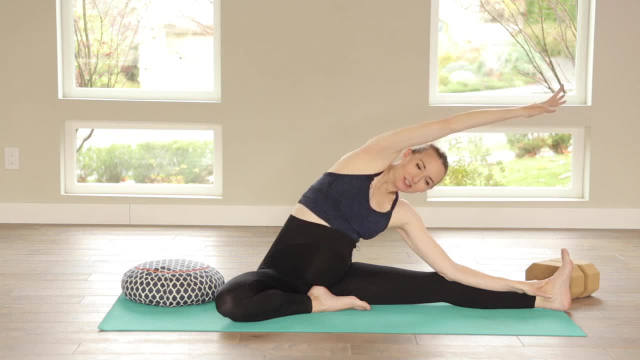 And this is a great place to hang out. And again, you can pull your hands together if you want to. You can put your hands together here and then pull your heels together, See if you can tap into a stretch On the right side of the low back. 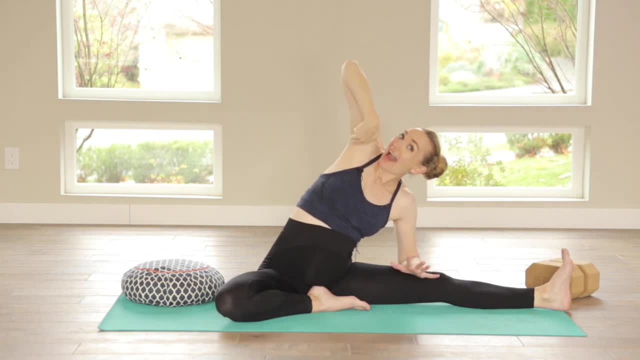 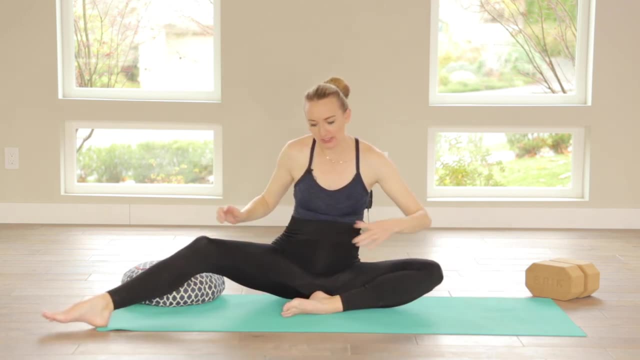 And this is a great place to hang out and stay a lot longer. I feel a huge stretch along the whole back seam of my body up through my side waist with this particular stretch. so let's do that exact same stretch on the other side. so see how I'm just swapping the legs out. so just do the other side. 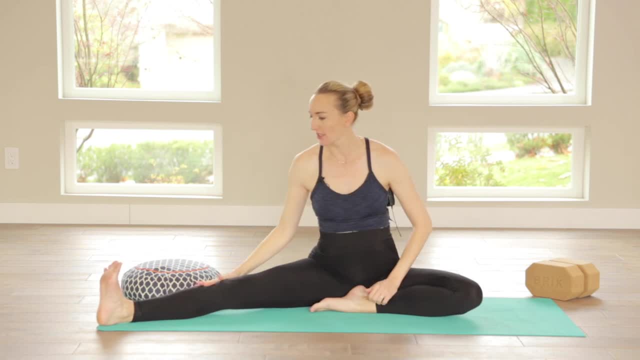 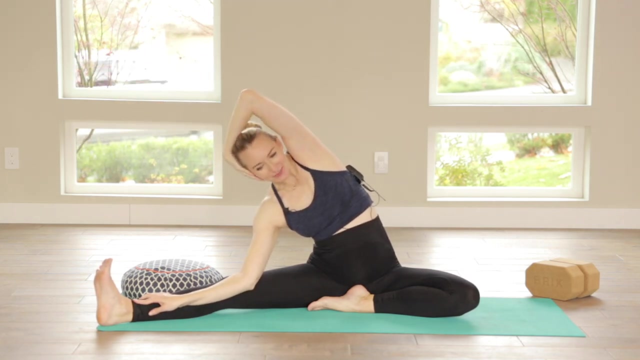 we'll do the open hip and then we'll do the closed hip to close foot flexed on the leg, that's long inhale reach. and come into this big side stretch option to take what I call the ear muff. so hand cups, the underside of the face or ear. 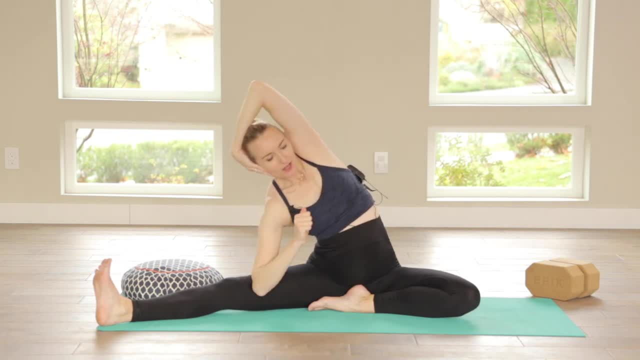 figure out where you want that bottom elbow and then remember it's not about touching the foot or how low you can get to your leg. we're kind of trying to torque. it's like you torque the upper body towards the ceiling while leaning over and now you're looking for a really deep stretch in the left low back and 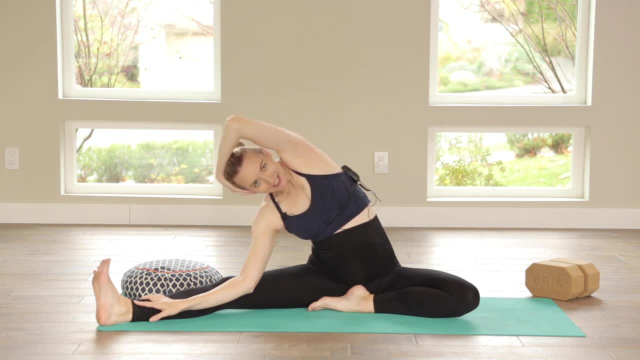 side waist. it's kind of like where you're you're looking for a really deep stretch in the left, low back and side waist. it's kind of like where you're booty connects up into your sideways, that sort of line that we're breathing into here. breathe in and out through the nose, try to cultivate the inhale and 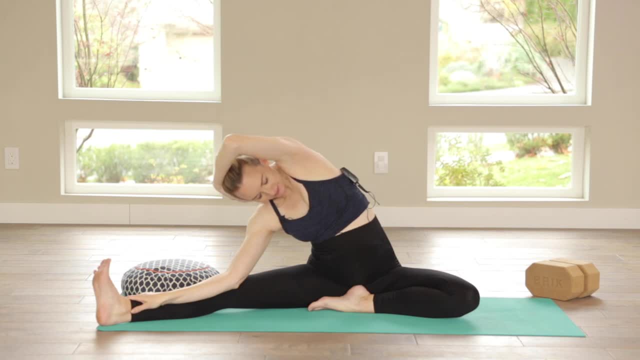 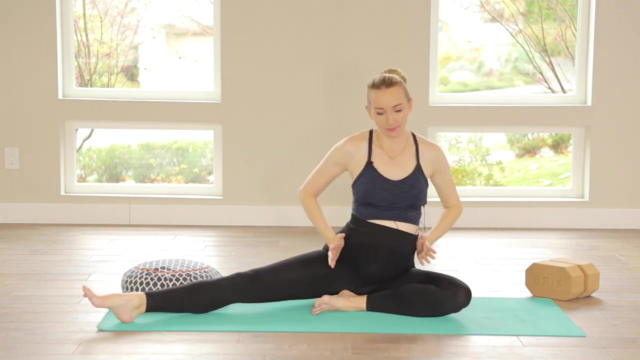 exhale to be equal in length. exhale to be equal in length. find that bottom hand, that bottom arm. you use it to support you as you come up. take both hands behind you, and now we'll shift. so, instead of the hips being kind of more open towards the side of the mat, we're really going to face the 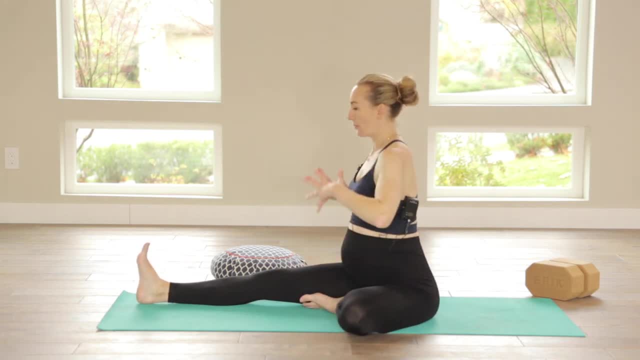 short end of our mat and then same stretch we did before before Inhale, reach up, get tall, Exhale, fold forward, Don't hold the foot, Draw the shoulder blades down the back And again you're just thinking of the heart moving forward towards. 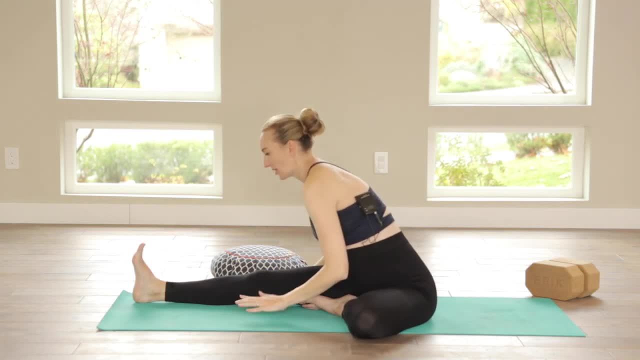 the knee, but with less of a focus on a stretch in the back of the leg. You could even bend your leg. We're more interested in opening up the low back and the back body. Dip the chin so the head is in line with the rest of the spine. 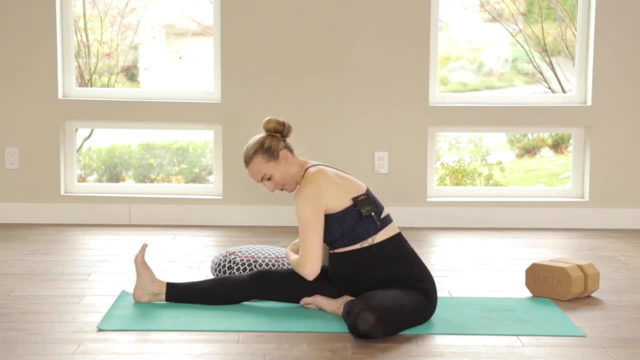 And I sometimes visualize like if my heart was a flashlight. instead of even pointing towards my knee, it's going a little bit off to the side, So more towards, like the pinky toe side of my foot is where it would be aiming for. So I'm coming into like a teeny, tiny bit of a twist. It's not. 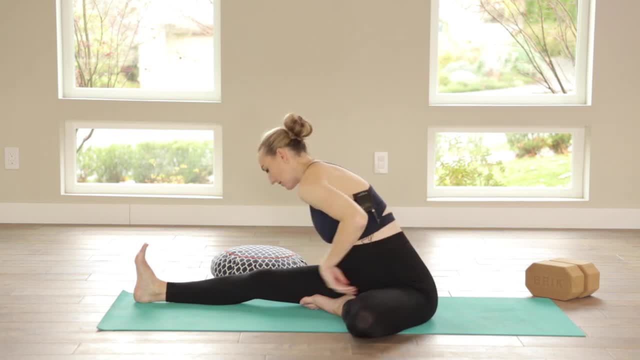 a real twist. It just kind of helps open up, I find, through the back side, waist a little bit more And relax the jaw, Relax the tongue, Send the breath down into the sacrum and low back, So really challenge your breathing to. 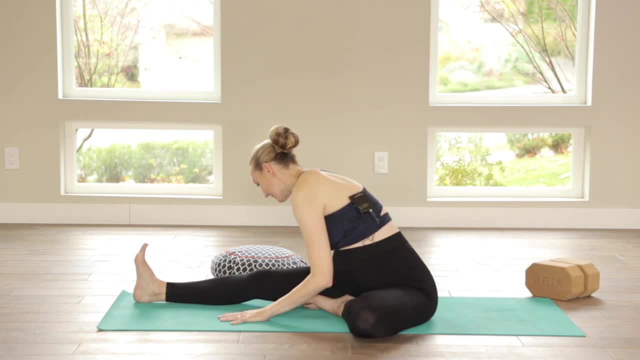 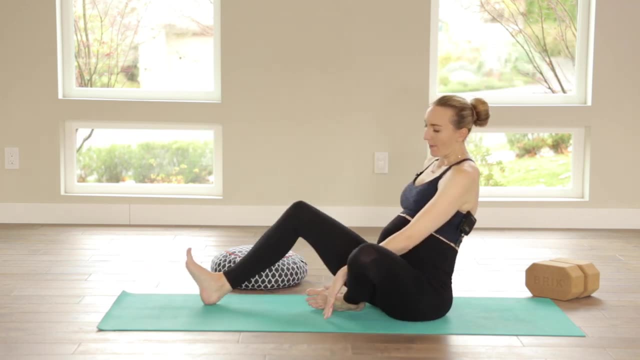 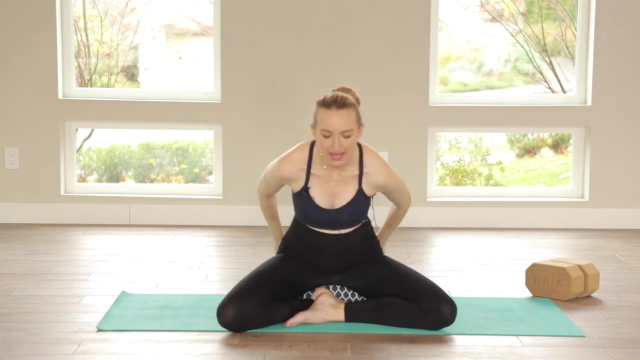 get bigger. That's going to really help with all these exercises. Good, And then press the hands into the floor, Slowly, come back To a cross-legged seat or however is comfortable for you, And just take three deep breaths to close. 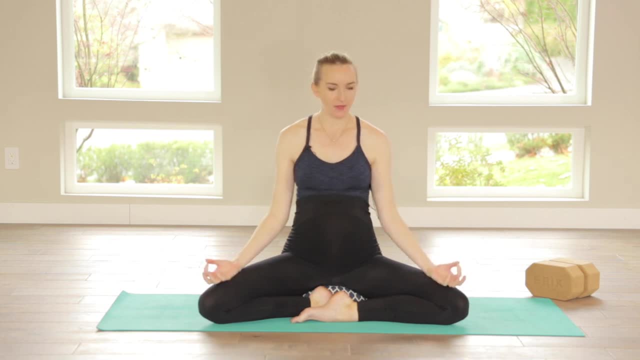 this little stretching session So you can have the palms face up on the thigh, index finger and thumb. touch heart gently, lifting, inhaling, exhaling, fully, breathing in, Breathing out Last time, Fill up with breath, Send breath down into the belly, into baby's home. 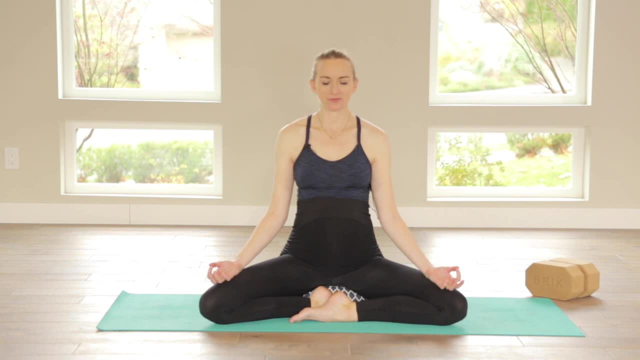 Complete exhalation And then bring the hands to prayer. I hope you feel a little bit better after practicing these stretches. Come back to this routine often And I'm sending you so much love From my heart to yours, namaste.